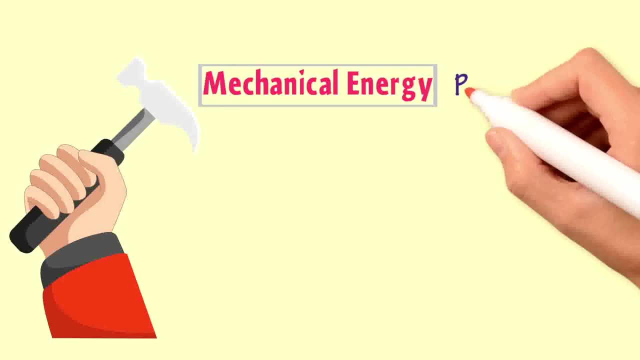 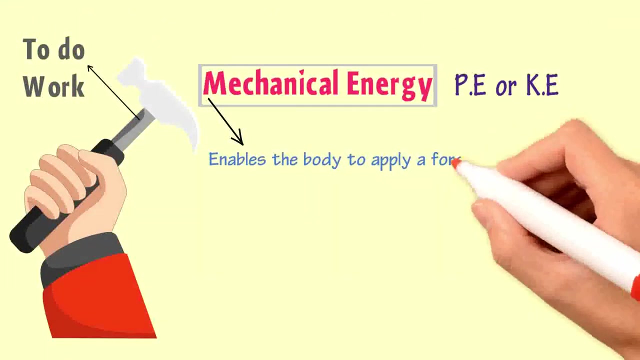 mechanical energy or mechanical energy, Whether it is in the form of potential energy or kinetic energy, is able to do work. It means that mechanical energy enables the body to apply a force to another body in order to displace it from its main position. Various examples can be: 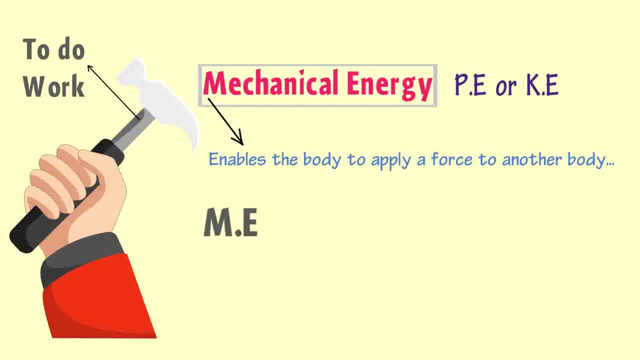 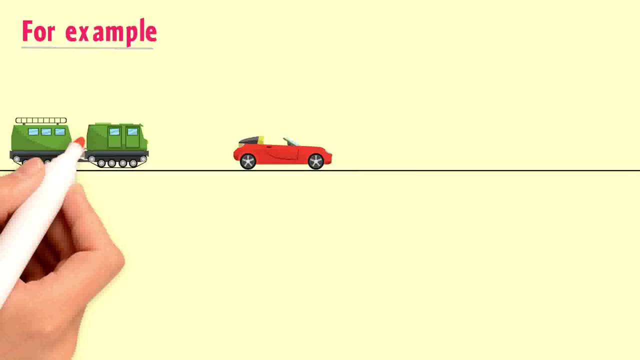 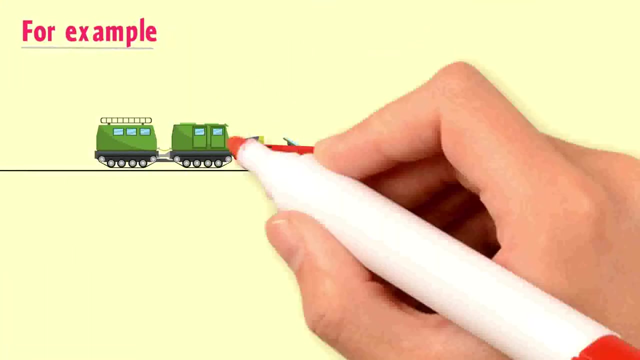 given of how a body can displace a force from its main position, of how an object with mechanical energy can harness that energy in order to apply a force to cause another object to be displaced. For example, if a fast-moving object hits a stationary object during collision. the mechanical energy of a moving object 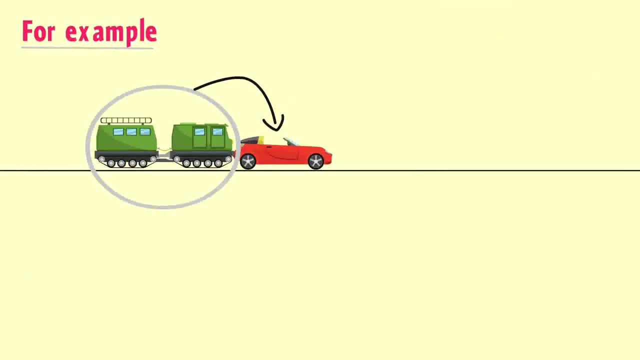 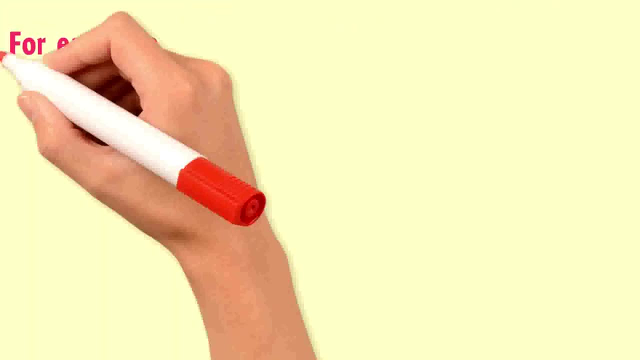 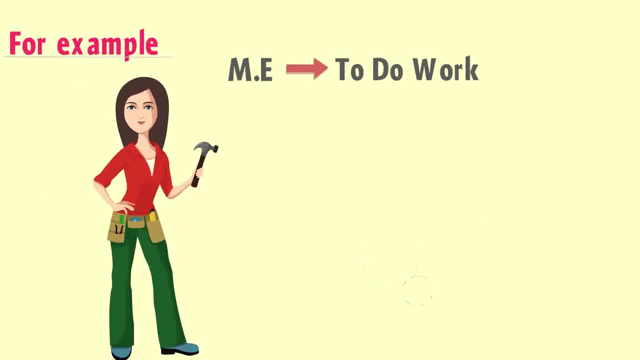 will cause the stationary object to move in the direction of exerted force. Another example that shows how mechanical energy is the ability of an object to do work is a hammer, For example. a hammer is a tool that utilizes mechanical energy to do work. 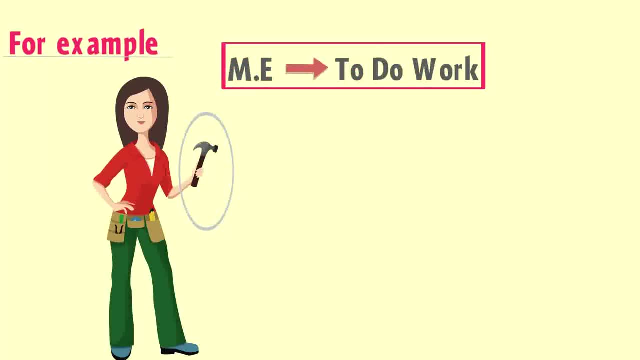 The mechanical energy of a hammer will cause the stationary object to move in the direction of exerted force. The mechanical energy of a hammer gives the hammer its ability to apply a force to a nil in order to cause it to be displaced, Because the hammer has mechanical energy. 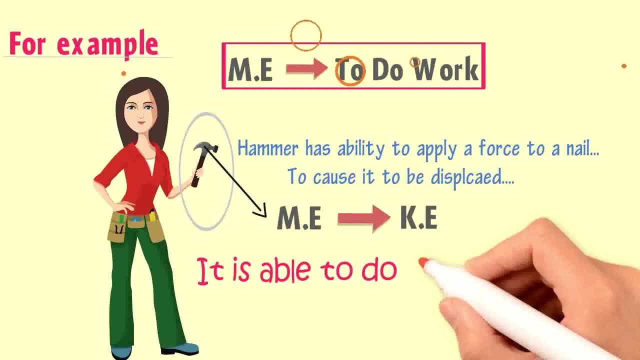 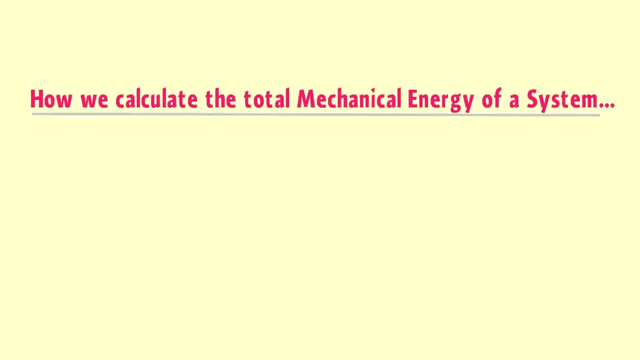 in the form of kinetic energy, it is able to do work on the nil. Therefore, mechanical energy is the ability to do work. Now, how can we calculate total mechanical energy of the system? As I mentioned earlier in the lecture that the mechanical energy can be the result of its motion, 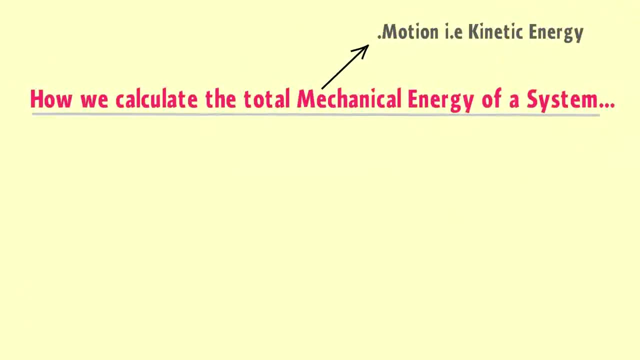 For example kinetic energy, are the result of its stored energy, of position, for example potential energy. Hence the total amount of mechanical energy is the sum of potential energy and the kinetic energy. ThatÕs why we write TOTAL MECHANICAL ENERGY IN THE기가.